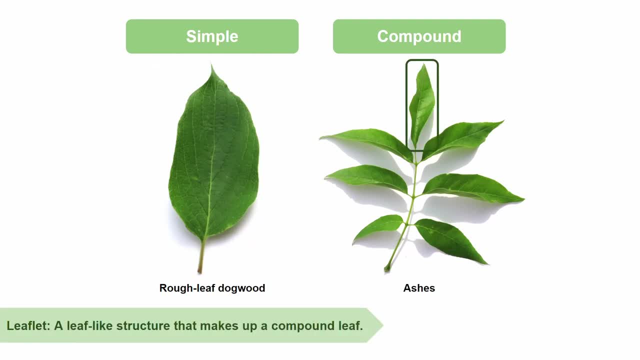 have multiple small leaflets per leaf blade. If you look at our example compound leaf, it has seven total leaflets. A leaflet itself is a leaf-like structure that makes up a compound leaf. Now what about our little nubs at the ends of the leaves? Those are the petioles, which is the part of the stalk that 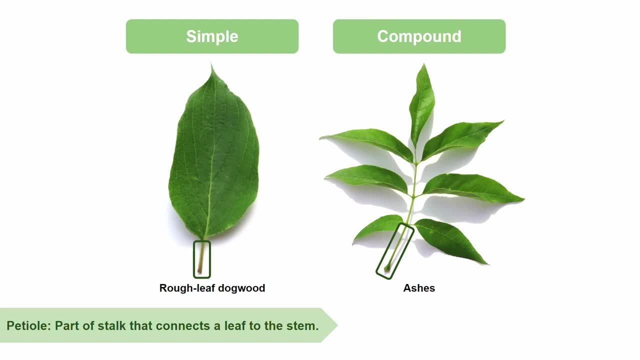 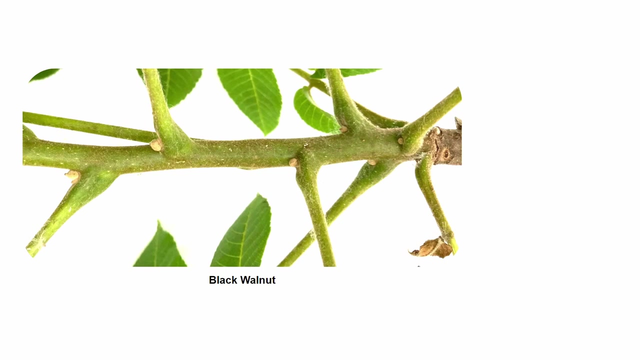 connects the leaf to the stem. Both simple and compound leaves have petioles. however, only compound leaves have a rachis, which is the point on a compound leaf where the leaflets meet. A helpful way to determine if you have a simple or a compound leaf is to look for a bud. 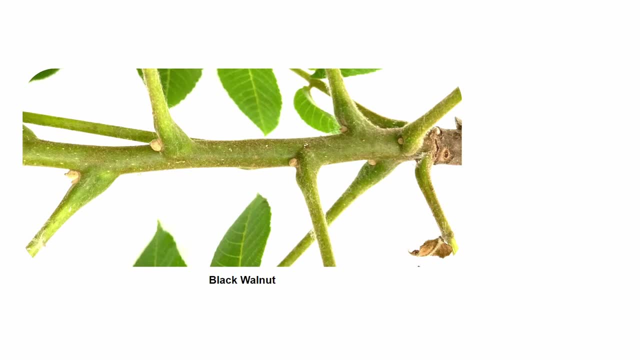 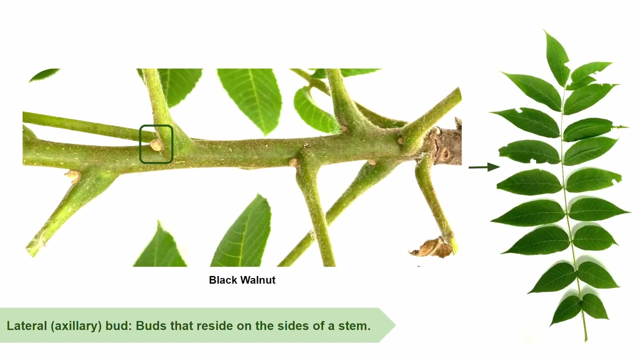 Here we have a photo of the stem of a Juglins nigra, otherwise known as black walnut. In this photo we can spot multiple lateral or auxiliary buds, which are buds that reside on the side of a stem. A whole leaf will emerge from a singular bud If the leaf is 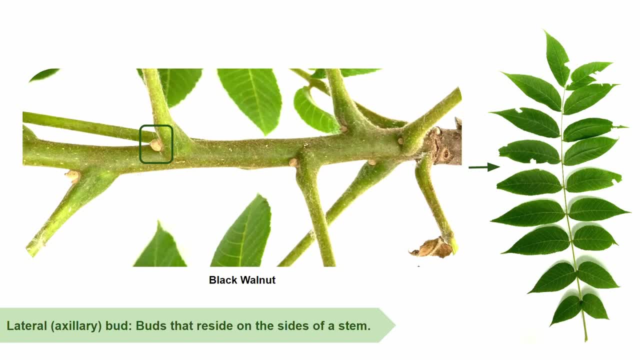 compound like the leaf right here, all of the leaflets will come from one bud. If you find a single leaflet- or in general we青 all leaflets to have two buds- we can identify which leaflet is where the bulb has to end and name that new leafbulb. Or if you have agelias lucky, 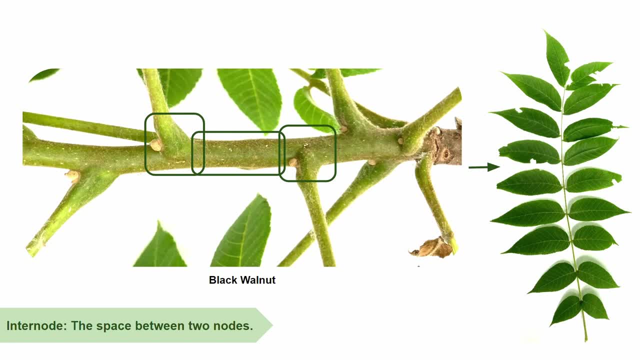 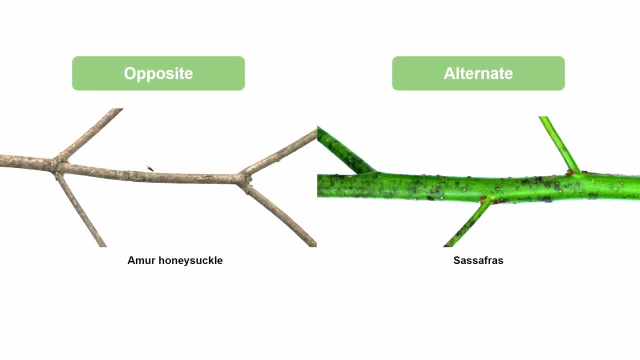 bud would be placed on the centre front, left side of the stem. By last time I tried, I lessened the or lamina. the leaf is simple. Determining if a tree has opposite or alternate leaves is a very important step in species identification. Lonicera macchi, otherwise known as a myrrh honeysuckle. 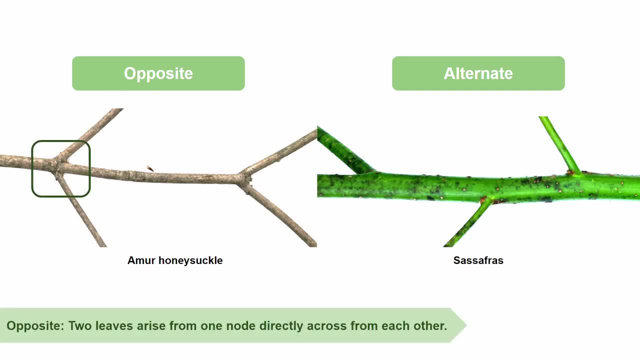 is a species that has opposite leaves. An opposite leaf pattern is seen when two leaves arise from one node directly across from each other. On the other hand, Sassafras albidum or the Sassafras tree, has an alternate leaf pattern. An alternate leaf pattern is seen when one leaf arises from: 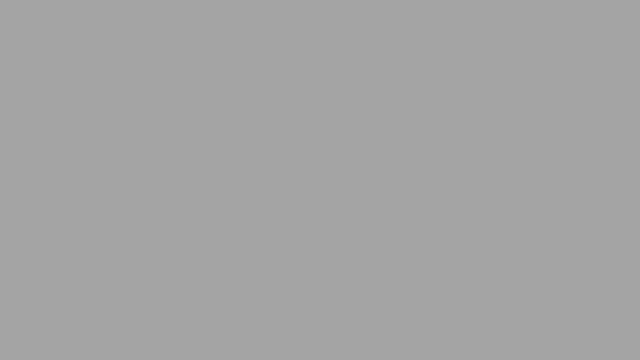 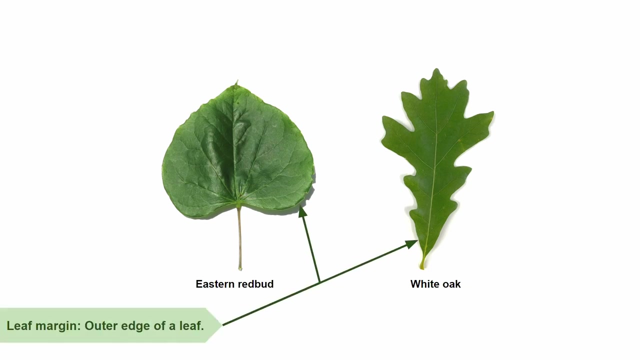 each node in an alternating pattern. Okay, enough with the stem, Let's move back to the leaves themselves. Let's start with leaf margins. A leaf margin is the outer edge of a leaf. There are two main categories, which are entire and lobed. Circus canadensis, otherwise known as eastern redbud. 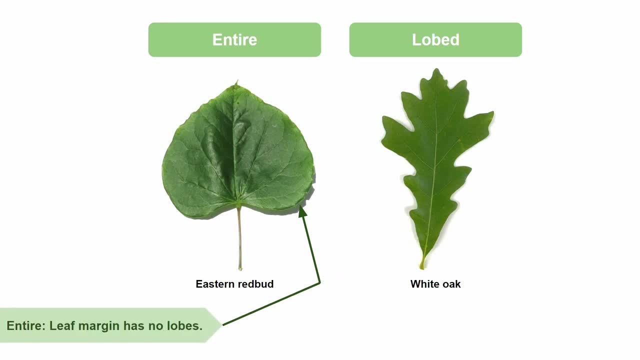 is entire, which means that its leaf margin has no lobes, whereas corcus alba, otherwise known as white oak, is lobed, which means that its leaf margin contains projections that extend from the center of the leaf. Now let's dig a. 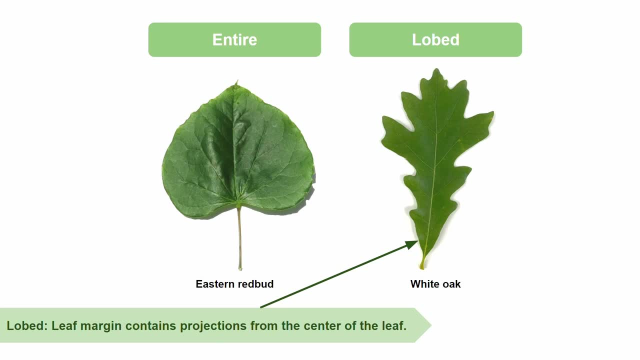 little deeper into lobed leaves and talk about lobes and sinuses. We already know that a lobe is a projection that extends from the center of a leaf, and if we take a look at our white oak leaf, we'll see that it has nine lobes. Sinuses, on the other hand, are the indents in the margin. 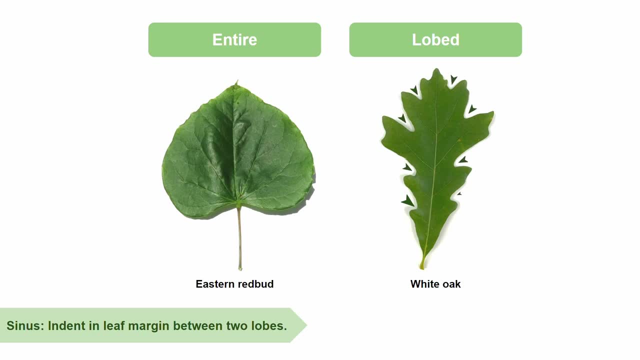 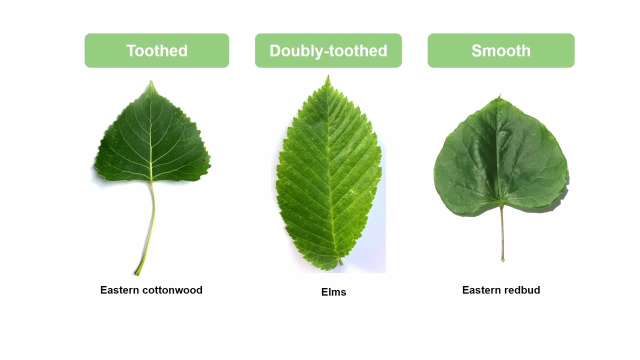 between two lobes. If we take a look at our white oak leaf, we'll see that it has nine lobes. On our white oak leaf there are eight sinuses. Besides being entire or lobed, leaves can be toothed, otherwise known as serrate, or they can be smooth. When a leaf is toothed, its margin has. 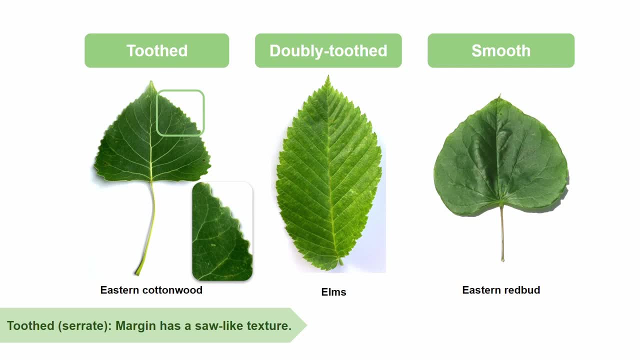 a saw-like texture to it. An example of this would be Populus deltoides, otherwise known as eastern cottonwood. We can take it a step further, though, and look at a leaf that is doubly toothed. To be doubly toothed, the teeth of the margin have a saw-like texture themselves. An example of this is: 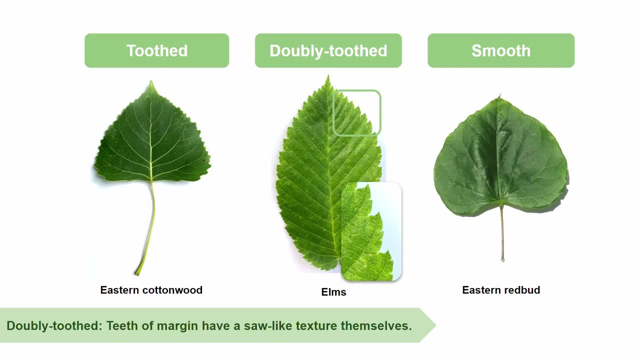 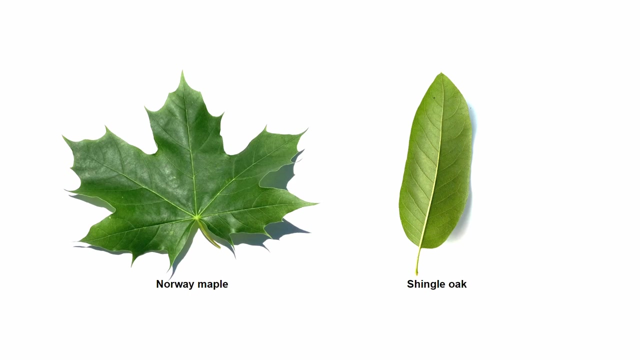 an example of a genus with doubly toothed leaves would be Ulmus, otherwise known as elm. Lastly, for smooth leaves, there are no teeth present on the leaf margin. An example of this would be the eastern redbud. Veining patterns are also helpful in leaf identification because they influence the 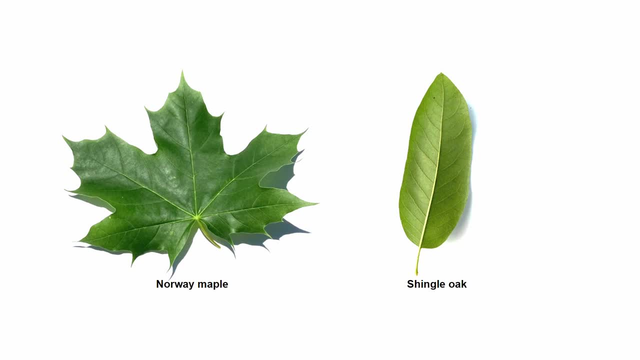 overall shape of the leaf. There are two main types of veining patterns for simple leaves that are super important to know. The first veining pattern is palmate, which looks like if you were to put your hand out in front of a leaf. you would be able to see the leaf If you were to put your hand. 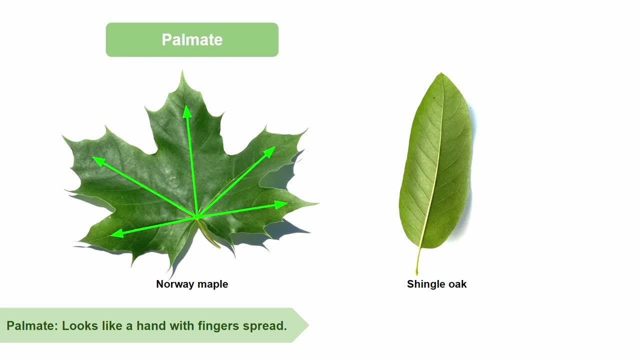 out in front of you and spread your fingers. Acer platinoides, otherwise known as Norway maple, is a very well-known tree that has a palmate veining pattern. The next commonly found veining pattern is pinnate, which resembles a feather and has similar parts on either side of the mid-vein. 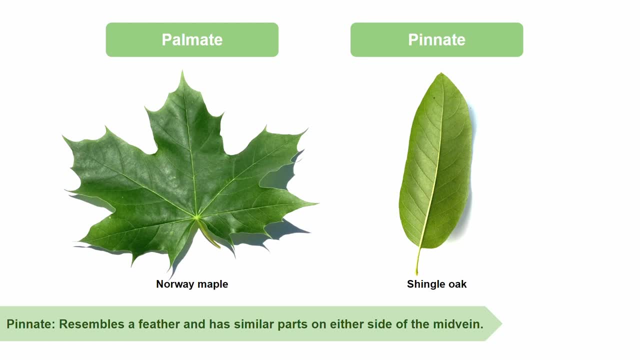 Quercus imbracaria, otherwise known as shingle oak, is a good example of a pinnate veining pattern. Now, the mid-vein is a central vein of the leaf. that is the center of the leaf, If you. 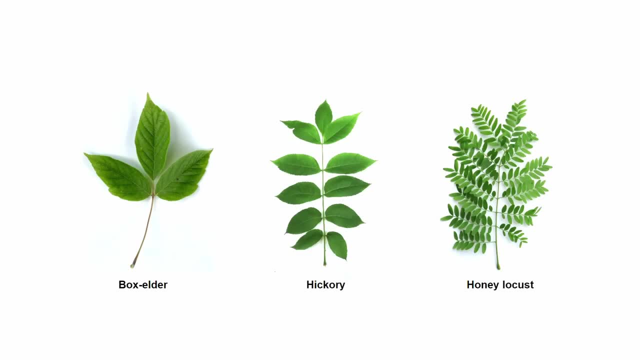 are using a pinnate veining pattern, you would want to make sure that the secondary veins will come from Like simple leaves. compound leaves can also be palmate or pinnate. Instead of being connected, the leaflets make up the hand or feather shape. Acer negundo, otherwise known as box elder. 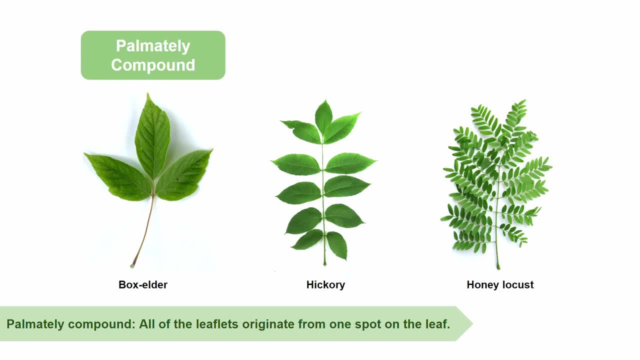 is a fairly common species, that is, palmately compound, which means all of the leaflets originate from one spot on the leaf. We can see that right here. If we imagine this leaf as a hand, it would only have three fingers because there are only three leaflets. On the other hand, the leaflets 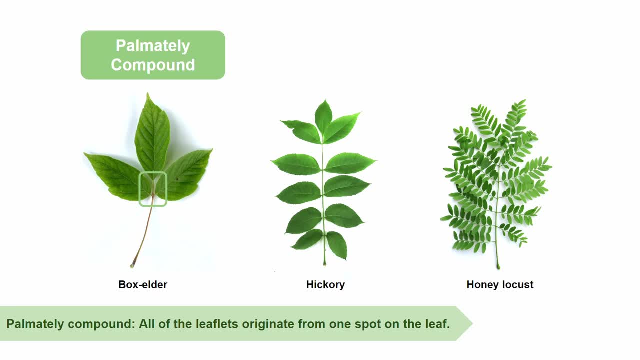 that are arranged on either side of the rachis. Now we can take this a step further, because some leaves are bipinnately compound, which means that each of the leaflets is divided again into more leaflets. I know it's a lot of leaflets. An example of a tree that is bipinnately compound. 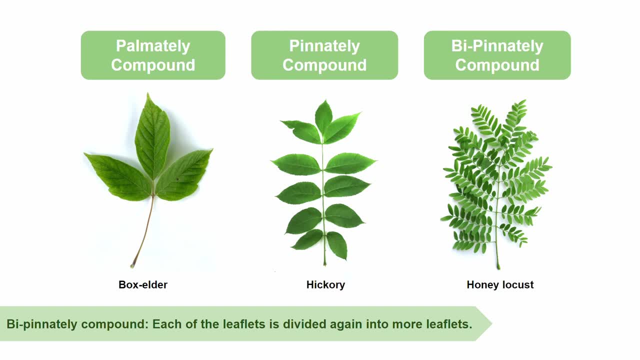 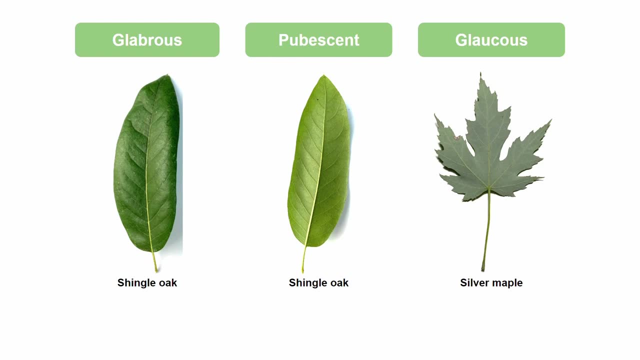 is Gleditia triacanthos or the honey locust tree. As we've seen, there are a lot of small ways to differentiate between leaves. There is, however, another way. That way is to see if the leaf is glabrous, glaucus or pubescent. A glabrous leaf is one that is hairless. An example. 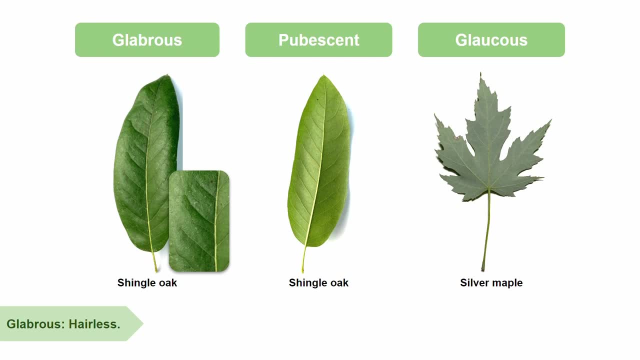 of a glabrous leaf is the top of our friend shingeloak. However, interestingly enough, the bottom of a shingeloak leaf is pubescent, which means that it is hairy or fuzzy. Now that we're familiar with glabrous and pubescent, it's time to tackle glaucus. A glaucus leaf is an outer leaf that is flat in shape. It's an outer leaf that is flat and flat and is located on an end. You should not be able to see the bottom of a leaf. It is just a small leaf. 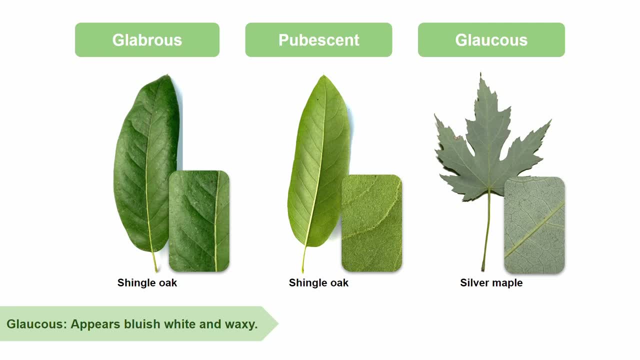 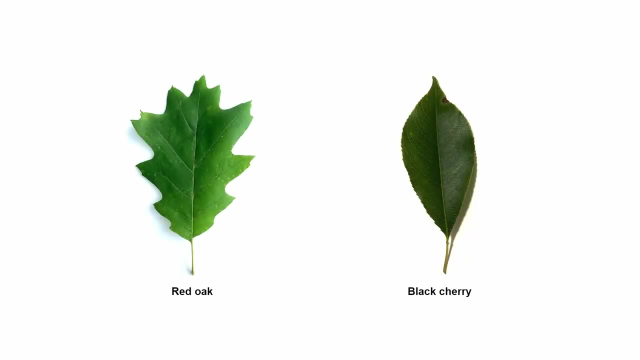 leaf is one that appears bluish, white and waxy. An example of a glaucus leaf would be the underside of an Acer saccharinum, otherwise known as silver maple leaf. You can see that it has that pale coloration to it. There are some additional traits that leaves may have that we, as plant identifiers, 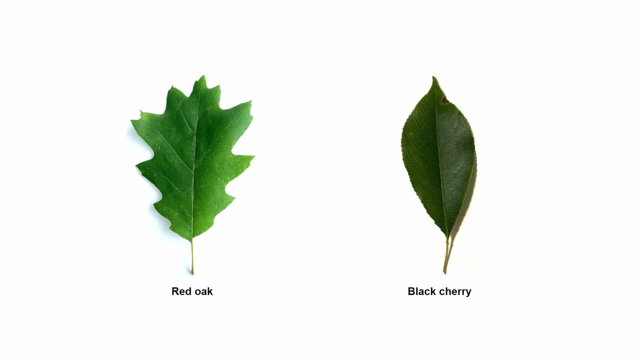 could put to use. Some leaves, like those of Corcus rubra, otherwise known as red oak, have bristles at the ends of their leaves. A bristle is a stiff hair that typically occurs at the end of a lobe. Another trait that is less common is glands. A species in my area that has glands is Prunus. 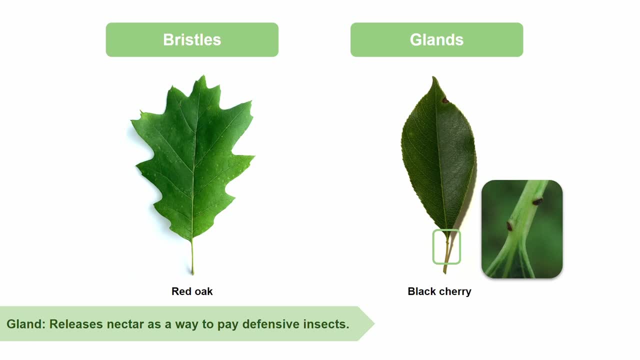 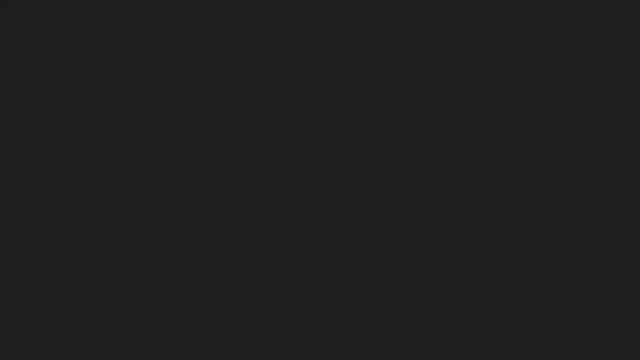 serotina, otherwise known as black cherry Glands, release nectar as a way to pay insects that eat herbivorous insects that could be harmful to the cherry tree. Stipules are a pair of leaf-like structures that grow at the end of a petiole. 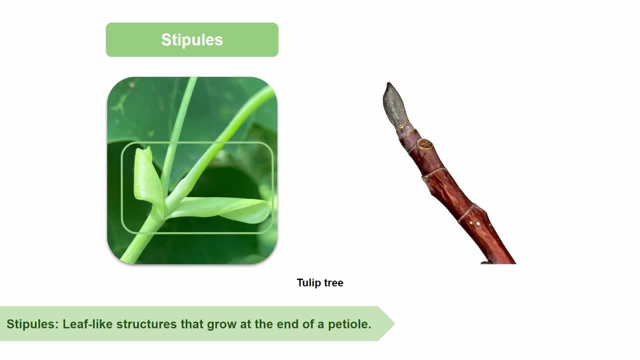 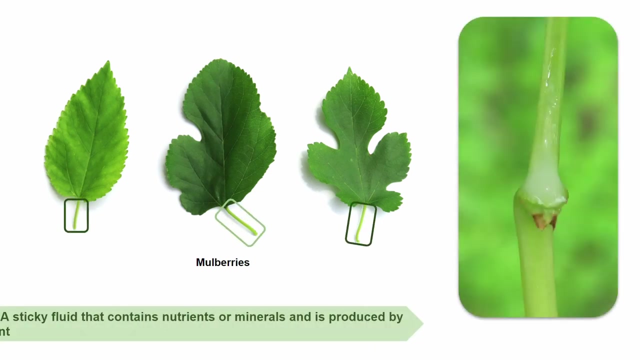 The stipules pictured are that of Liriodendron tulipifera or the tulip tree. After they fall off, they leave behind a stipule scar all the way around the twig. This can be useful for identifying the twig in the wintertime. Some species, such as mulberries, have leaves that leak a white milky. 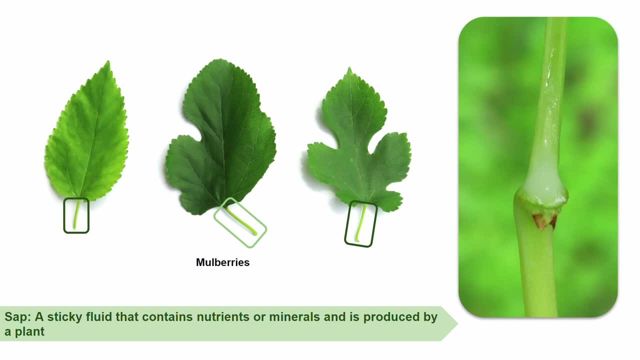 sap when they're broken. Sap is a sticky fluid that contains nutrients or minerals and is produced by a plant. This can be useful for identifying some plant species. All right, just for fun, we're going to do an example. Here we have an unknown tree species. 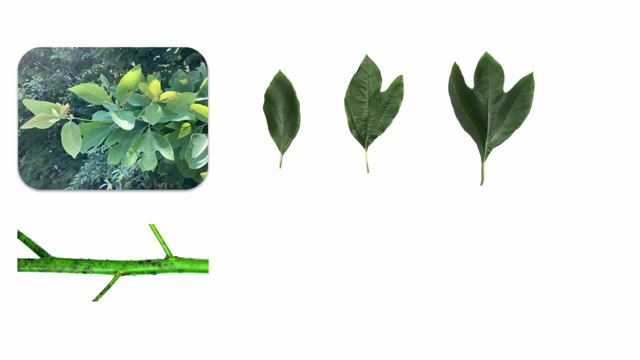 Some of you might already know what it is, but please don't shout it out. We're going to work through a series of questions to review what we've learned and together we will identify this tree. There are six main questions you should keep in mind when you're trying to identify a tree. 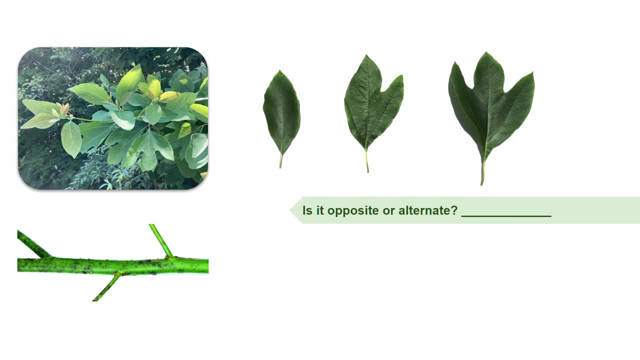 Is it opposite or alternate? Based on the section of the twig shown here, we can safely say that our tree is alternate because the leaves are attached in an alternating pattern. Are the leaves simple or compound? They'd be simple. They are not broken into leaflets. Are the leaves toothed? 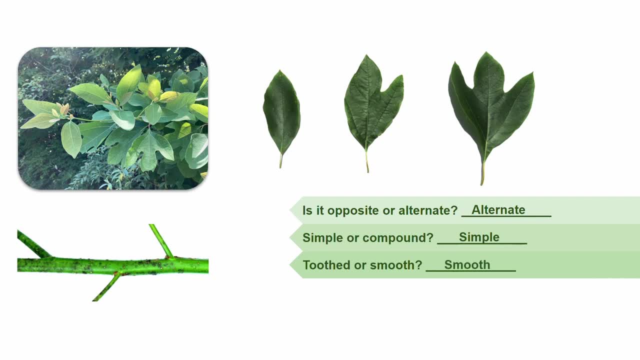 or smooth. They are smooth. The margin of the leaves don't have a saw-like texture. Are the leaves lobed or entire? These leaves are lobed. This particular species is interesting because it has three different leaf shapes. The first is single-lobed, which could be classified as entire. 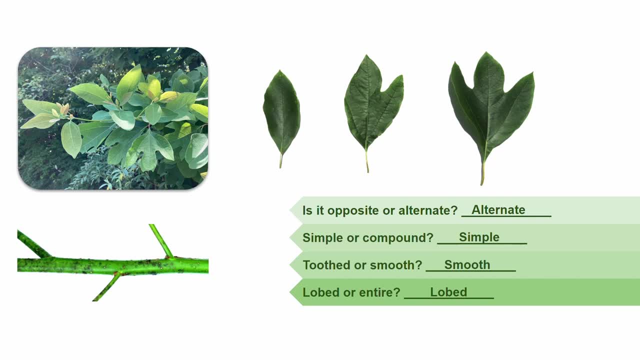 However, it also has two-lobed and three-lobed leaves All right. are the leaves glaucus, glabrous or pubescent? The leaves are glabrous, but they can also sometimes be slightly pubescent. 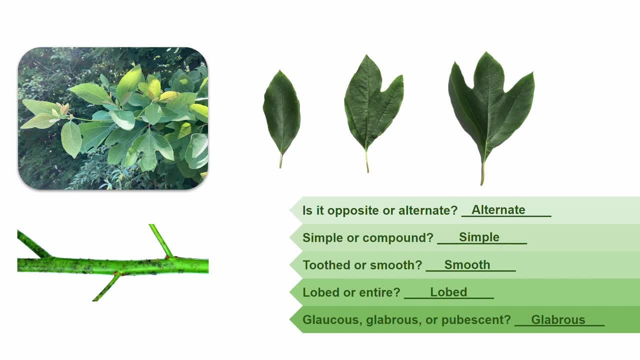 You wouldn't be able to see that from this photo, so glabrous- is the right answer. Lastly, does this species have any extra traits? It does, but it's one that we haven't talked about yet, so it was a bit of a trick question, so I'm sorry for that. Its extra trait is odor When you crumble the.